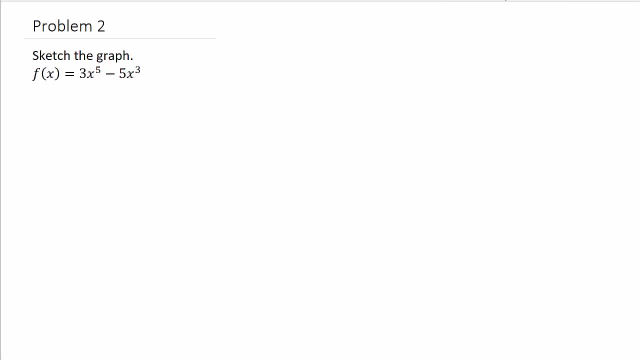 The intervals where the function is concave up and concave down, And then any inflection points. Alright, so first thing, let's go ahead and find where the function is increasing and decreasing. So to do that, we need to find the critical numbers. So to do that, you've got to take the first derivative, So that's 15x to the 4th minus 15x to the 5th. 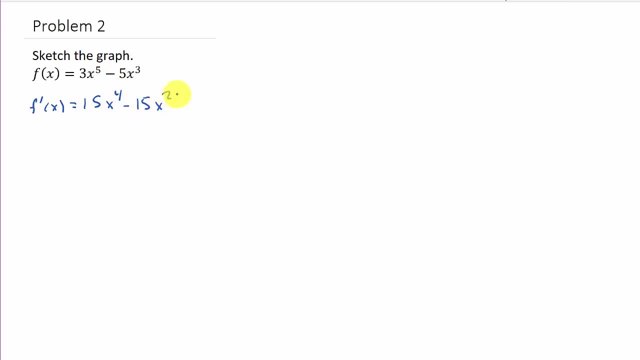 15x squared And then you set the first derivative equal to 0. And solve, So we'll factor out a 15x squared And then that's times, x squared minus 1 equals 0. So we get x equals 0 or x equals plus or minus 1.. 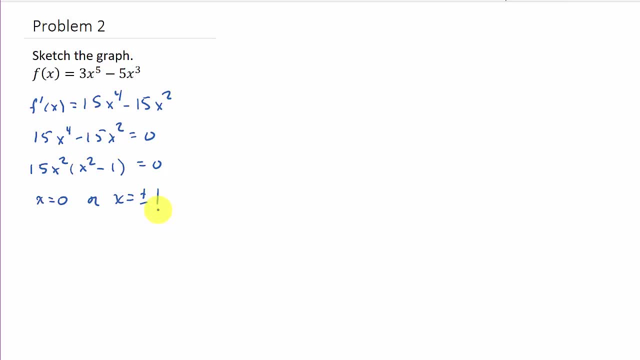 Alright. so Once you find your critical numbers, you take the critical numbers and you plug and you plot them on a number line. So we've got negative 1, 0, 1.. Alright, and we've got three critical numbers. So that's going to break the number line up into four regions. And then what I need to do is I need to choose a number. Alright, so we've got three critical numbers, So that's going to break the number line up into four regions, And then what I need to do is I need to choose a number. And then what I need to do is I need to choose a number. 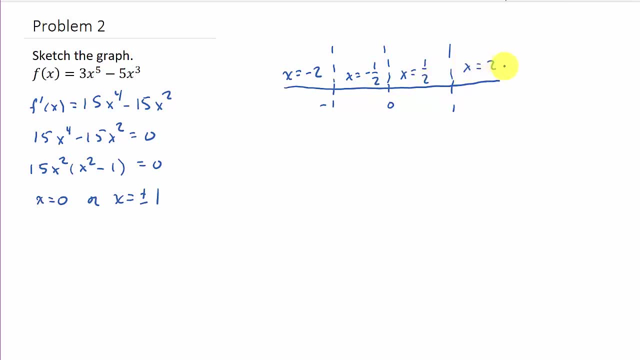 From each region. Alright, makes no difference what numbers you choose, just as long as you choose a number from each region, Alright. Now We have to take The first derivative. Let me erase that x there. Okay, so now we've got to take the first derivative. 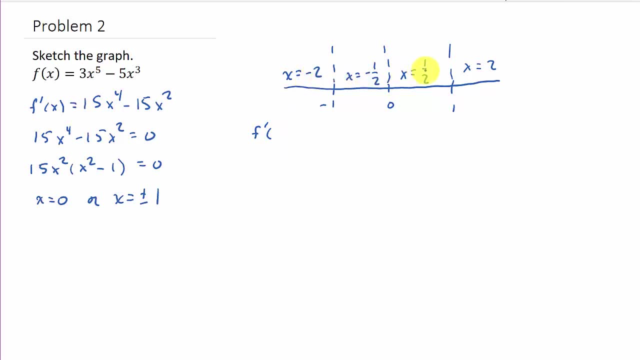 And evaluate the first, first derivative at each one of these X values. Okay, So you can take each X value, plug it in and get your Y value. Okay, But we don't care. We don't care about the exact Y value that we're. 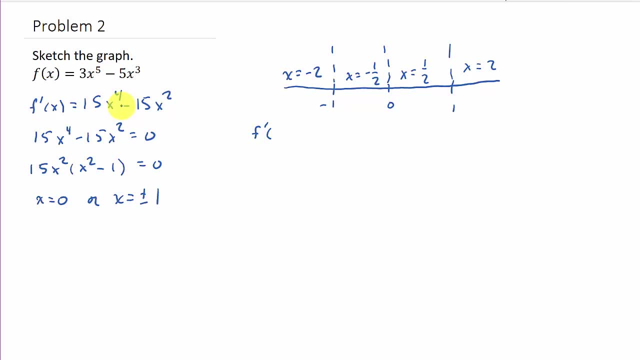 going to get. Okay, That makes no difference to us. All we care about when we plug each of these in. all we care about is it positive or negative. That's it, Okay. Now, what I want you to understand that this, this function here, is the same as this function. This one's just factored, Okay. 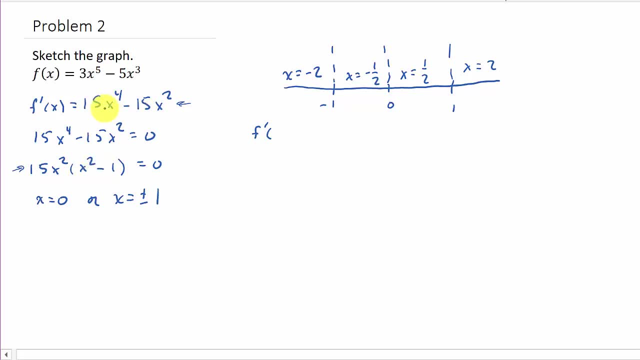 It's not factored completely, but it's factored out of 15 X squared. All right, So I'm going to plug this in negative 2 in. all right, so i can plug the negative 2 in, get a y value. but i don't really care about. 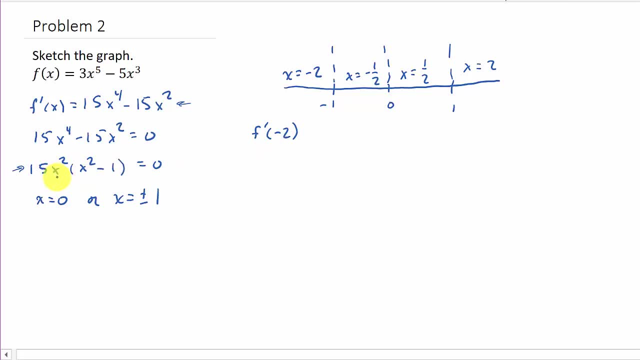 that. look, if i plug the negative 2 in here, that's negative. 2 squared is 4, 4 times 15. positive number: okay, 4 times 15, this is a positive. and then if i plug the negative 2 in here, that's 4 minus 1. 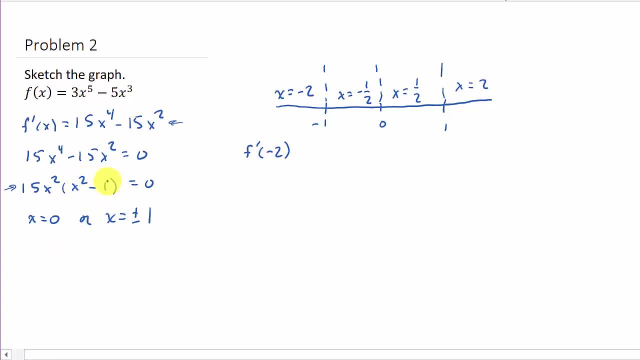 well, 4 minus 1 is positive. so this is a positive number here. this is a positive number here. so a positive times a positive is positive, so that's greater than zero. so what that tells me? since i took a number from this region, plugged it into the first derivative, i got a positive number. 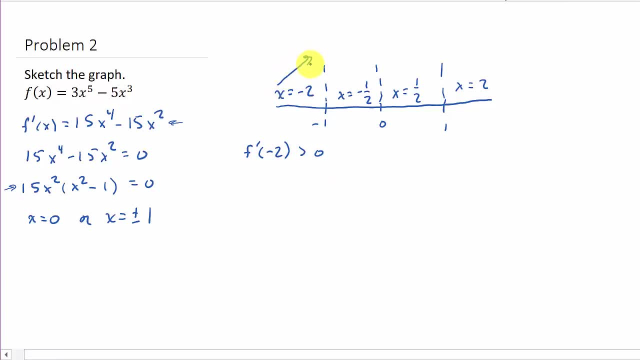 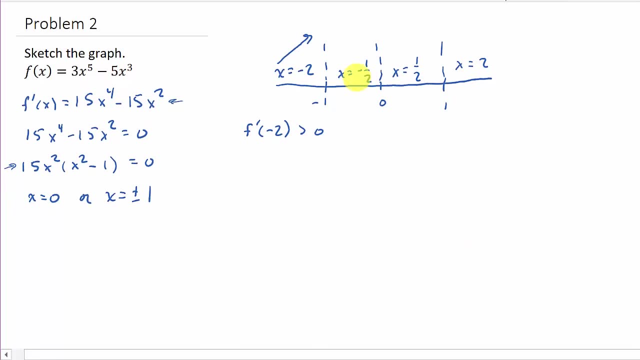 so that means the function's increasing on this interval. okay, now let's take the negative 1 half and plug it in, so i get negative 1 half squared. well, that's positive. so a positive times a positive, that's going to be positive out here. and then, if i take 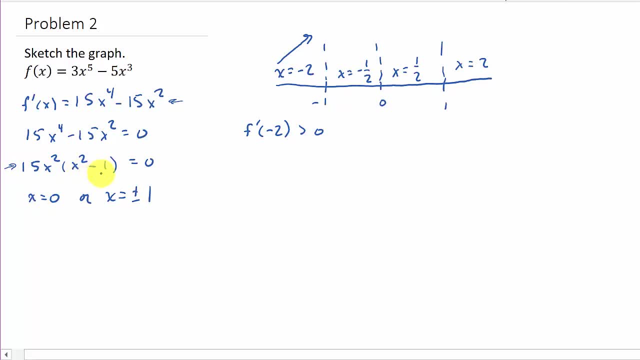 negative. 1 half squared, that's 1 4 1. 4 minus 1 is negative. so this is a negative times a positive, which is negative. let me go ahead and write that down. that's negative. and then i've got f prime of one half. so if i plug the one half into here, that's positive out here. 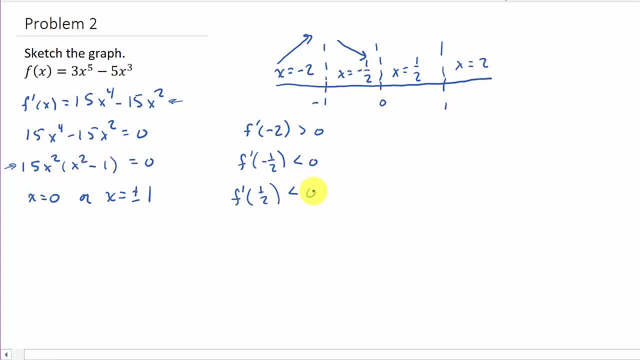 that's negative in here, so that's less than zero, so that means it's decreasing, okay. and then i do the f prime of two. if i plug the, if i plug the two in, that's positive. that's positive in here, so that makes the whole thing positive. so that means it's. 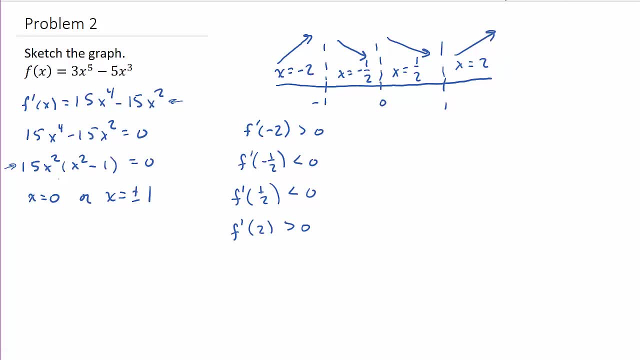 increasing. okay, so that tells me that this thing is decreasing: from negative one to one. okay, from negative one to one, it's decreasing, and then it's increasing from negative infinity to negative one and from one to positive infinity. see, it's increasing here and here. all right, so now. 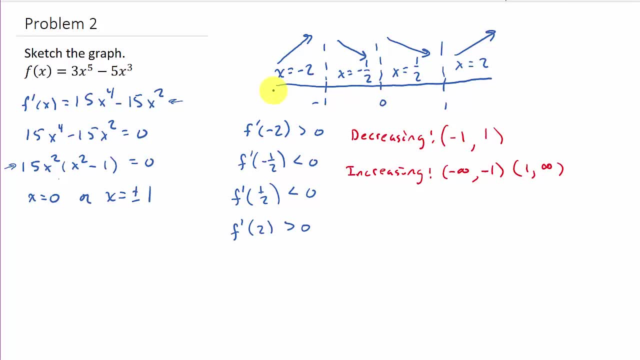 what we're looking for is we're looking for local max and minimum values. all right now, you notice i did this in red. what i would recommend that you do is when you're working these things, whenever you're finding increasing, decreasing, when you're finding your local max and 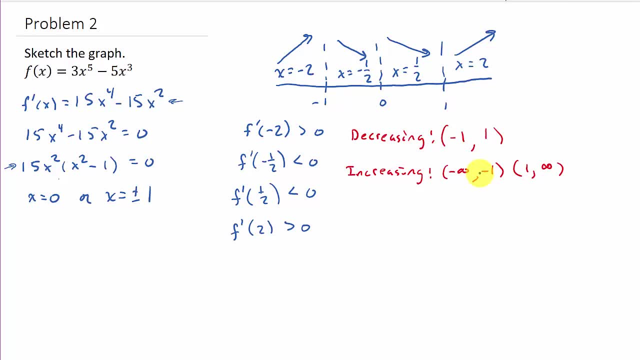 max mens, whenever you're finding the intervals of concavity and whenever you're finding inflection points, I would like for you, I mean, put a star beside them. I'm just writing them in different colors, but mark it, because you're going to use this to graph. Okay, So we found increasing and 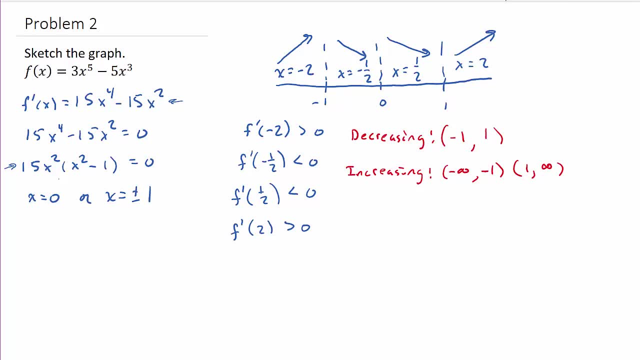 decreasing. Now let's look for local maximum and minimum values. All right, So the local maximum and minimum values. Well, if you look at this, you notice, on this interval here, this graph is increasing And then when it hits negative one, it starts decreasing. So look at that. That tells us. 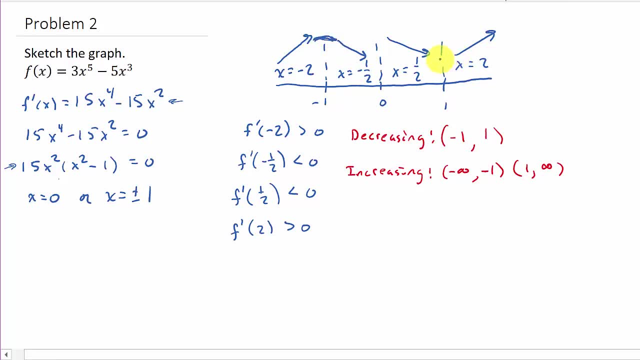 that's a local maximum. And then if you see here it's decreasing And then here it's increasing, Well that tells us at one we have a local minimum, but here it's not changing, It's decreasing. It's just decreasing the whole time. So there's no local max or men there. 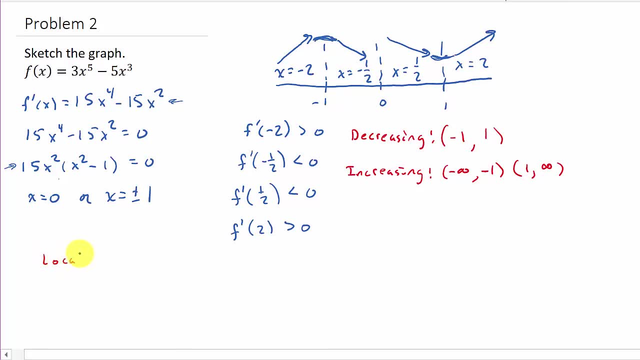 All right, So we have a local minimum at one. Okay Now, local minimum, local maximum. those are points on the graph. That's a point coordinate. So we need an X and a Y. Well, we've got the X coordinate. We've got that from here. That's one. Now we need the Y. 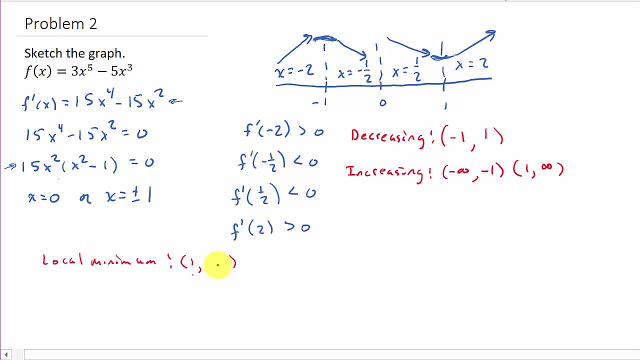 coordinate. So do you remember? when you have an X coordinate, how do you find the Y coordinate? Well, you take the X coordinate, you plug it back into the original function. One of the biggest mistakes students make is they'll take that one and plug it back into. 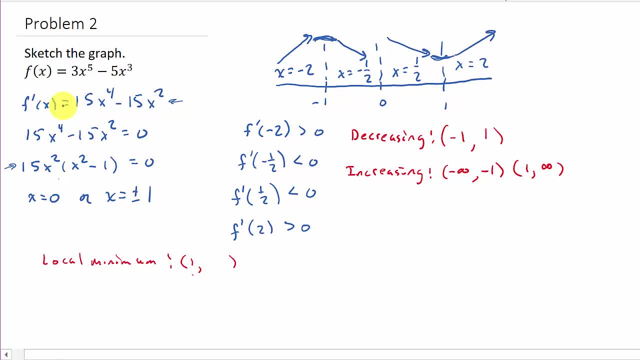 the derivative. You don't do that. You've got an X coordinate, You're looking for a Y coordinate, So you have to plug it back into the original function to get your Y coordinate. So that's going to give me: F of one is equal to three times one, to the fifth minus five. 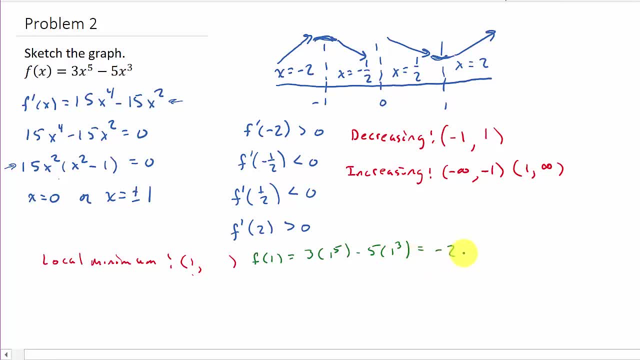 times one cubed, And that's just negative two. Okay, Yep, Three minus five, negative two. Then we have a local maximum. Well, here's your local maximum at negative one. And then we need the y coordinate. so we're going to take the negative 1, plug it back into the original. 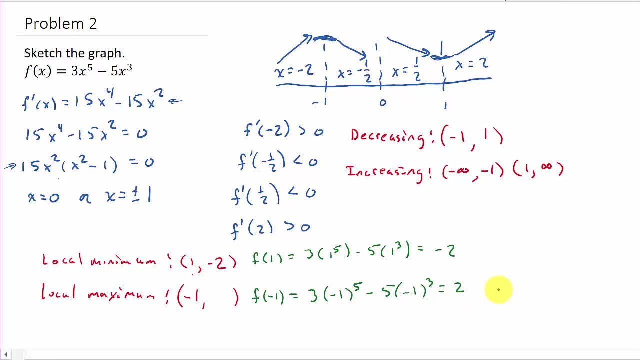 and that is going to give us- I believe that's positive 2.. Alright, so we found increasing decreasing, we found local max and min and now we're looking for concavity. Where is it concave up, where is it concave down? 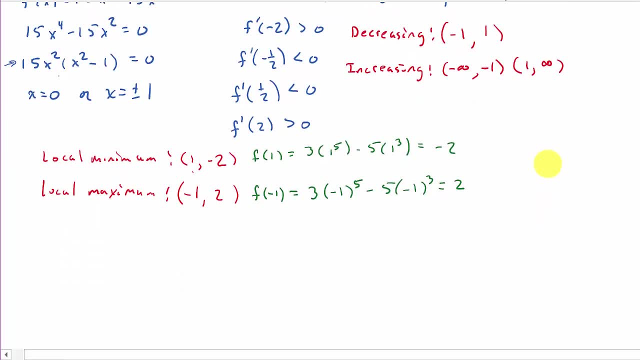 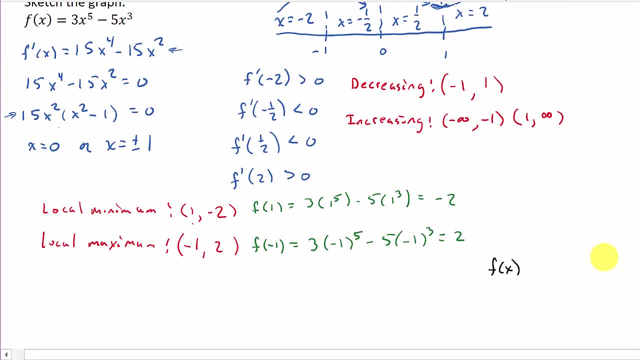 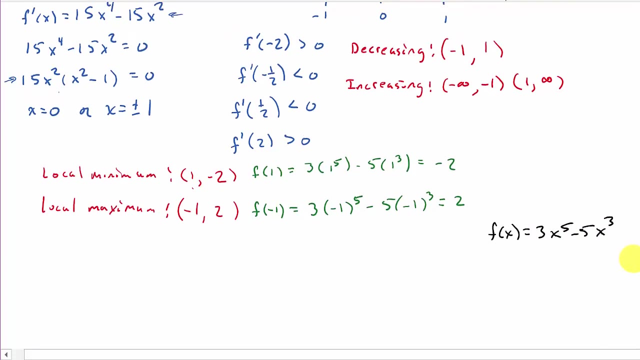 Alright, so let me scroll this up some, and what I'm going to do is right here, I'm going to rewrite the original problem, just so we can see it okay, and I'm going to leave it about right there for now. 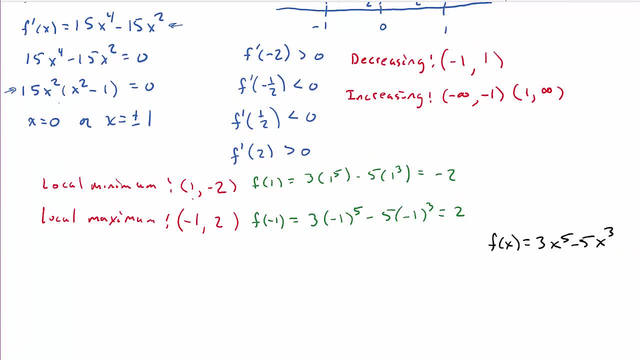 Alright. So to find concavity, We need the second derivative. So, if you remember earlier, if you remember earlier, here's our function. Well, we took the first derivative, which is this: okay, There's the first derivative, and so now to find the second derivative we've got to take. 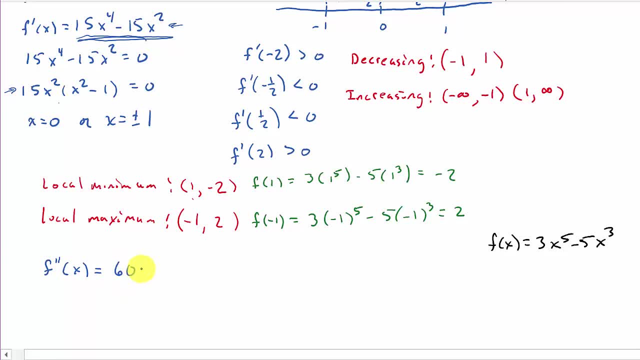 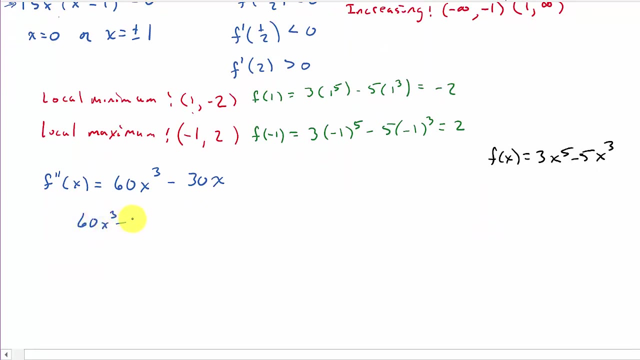 the derivative of this. So that is going to be what: 60x cubed minus 30x? Alright, Alright, Alright. You take the second derivative and set it equal to zero, So that's 60x cubed minus 30x equals zero. And so that's going to be 30x times 2x minus 1 equals zero. 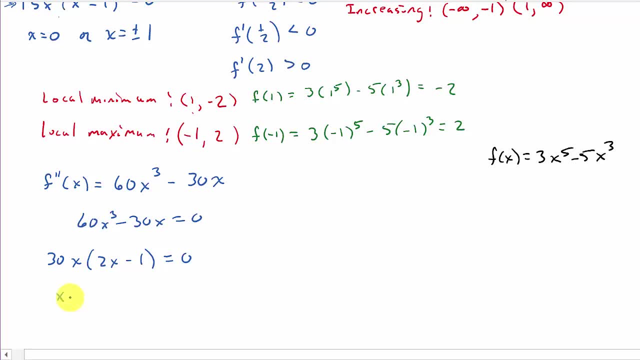 Alright, so this is going to give me x equals zero, or- and I'm sorry that should be 2x squared. Or that's going to give me x squared equals one half. So x equals plus or minus square root of 2 over 2.. Alright, so that's kind of nasty there, But it'll be okay. 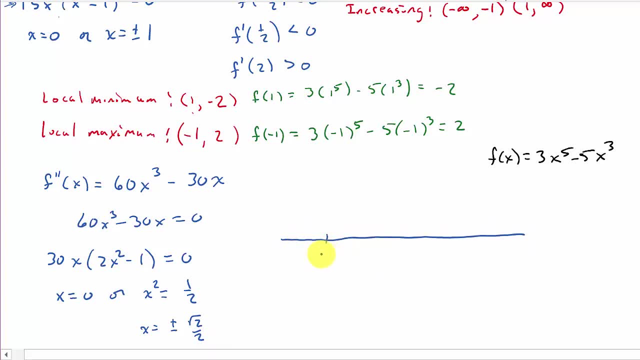 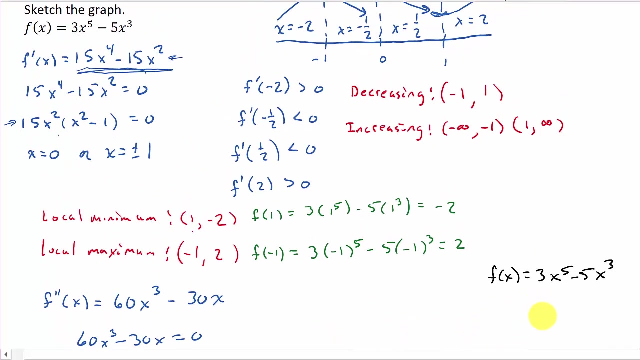 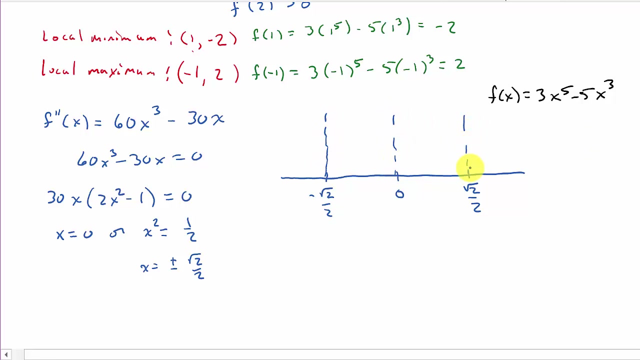 Alright, so let's plot this on a number. So we've got negative square root of 2 over 2.. We've got square root of 2 over 2.. And zero, Okay, So once you find the second derivative- Okay, You find the second derivative, You set it equal to zero, Solve for x And those values you get for x, you plot them on the number line, Just look, Just like we did up here. And then what that does is that breaks it up, In this case into four regions. 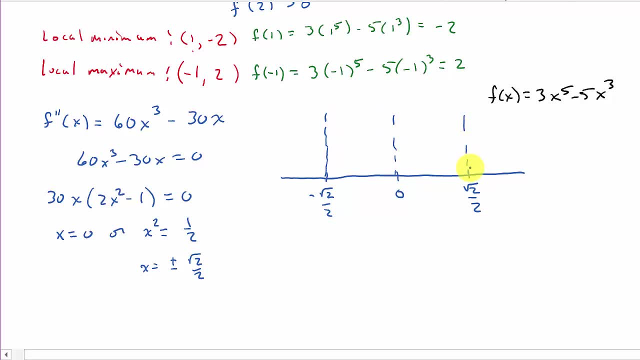 So we've got to choose a point from each region. So first let's see exactly what the square root of 2 over 2 is. That's .707.. Okay, .707.. So I can choose. x equals negative 1.. X is negative one half, X equals one half And x equals 1.. 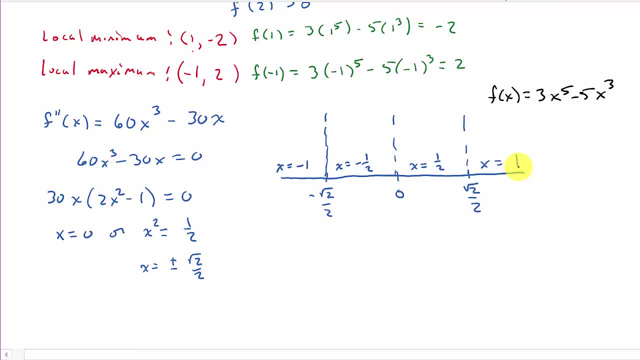 Alright. so now I have to evaluate the second derivative at each of these values here. So let's do f of negative 1.. So well, let's just plug it into the one that's factored To me. that's just easier to evaluate. 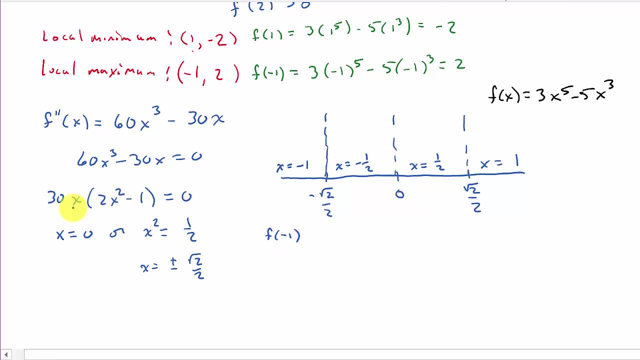 Well, so if I plug the negative 1 in, that's going to be what That's a negative out here, right, 30 times negative 1.. And then if I plug the negative 1 into here, that's 2 times negative 1.. 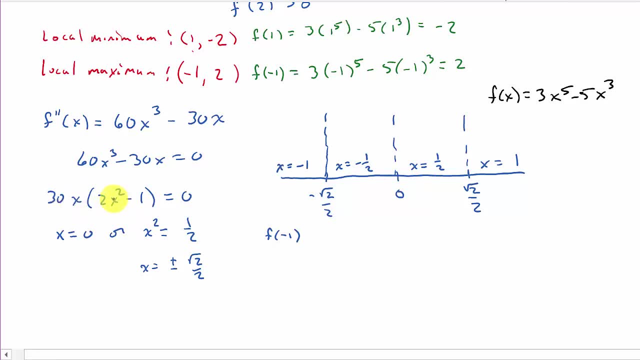 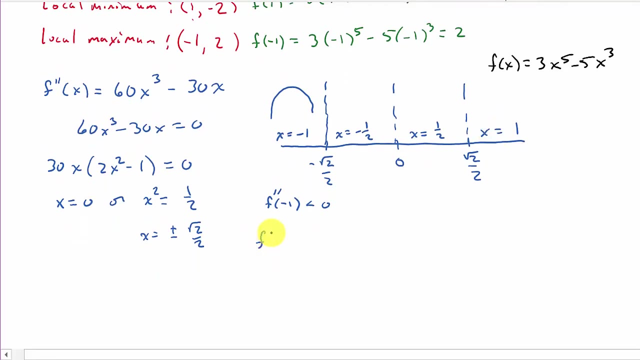 That's positive. So I have a negative times a positive. So that's negative, So that means it's concave down And I'm sorry that should be f double prime. And then I have f double prime of negative one half. So that's going to be a negative out here, And then if I plug the negative one half in, that's going to be what One. fourth: 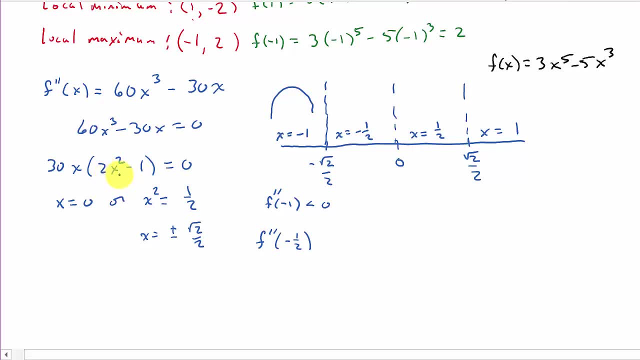 And so 2.. times one fourth is one half minus one, that's negative. so a negative times a negative is positive, and so that means here it's concave upward, and then we've got F double prime of one half. so if I plug the one half in, that's positive. 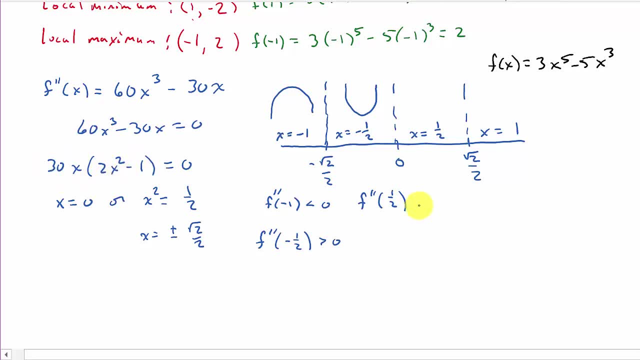 that's going to be negative in here. so a positive times a negative is negative. so that's concave down and then the F of F, double prime of one. that's going to be what a positive and a positive. so that's going to make it positive and so that's. 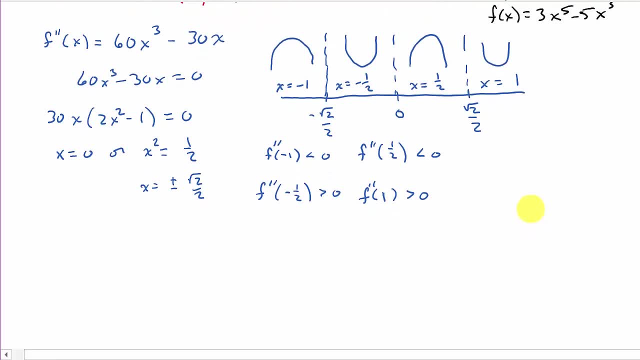 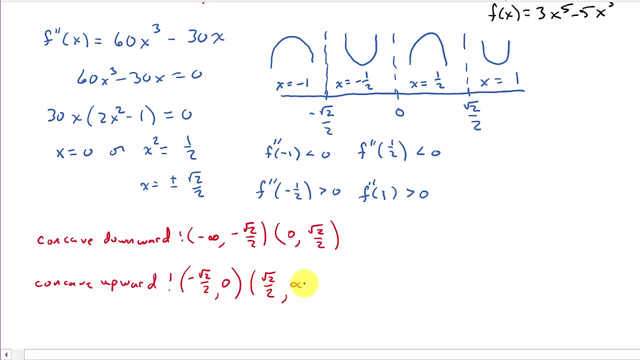 concave upward. and so that tells me it is concave downward from negative infinity to negative square root of 2 over 2 and 0 to square root of 2 over 2. and then it's concave upward from negative square root of 2 over 2 to 0 and square root of 2 over 2 to infinity. 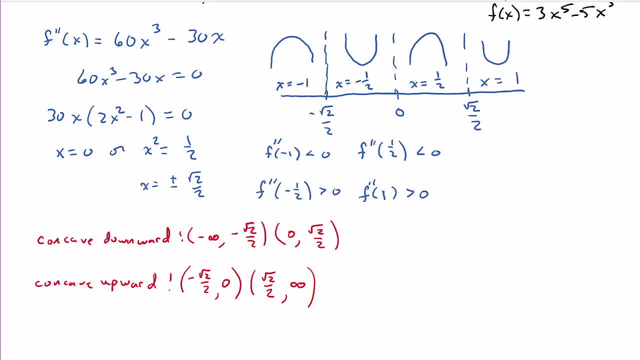 alright, now what we're looking for is inflection points. alright, so the inflection point. there are inflection points. that's where the graph changes concavity. ok, so that's what we're looking for. where it changes concavity. well, you can see it changes concavity at. 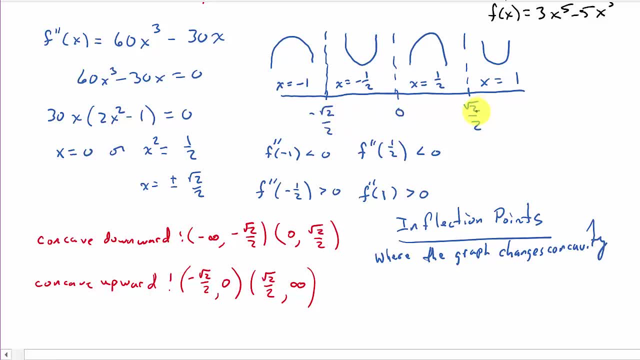 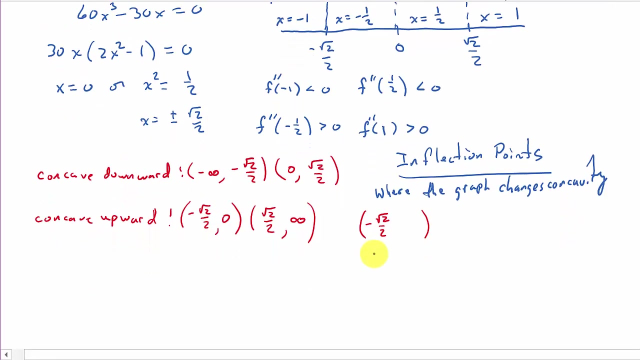 negative square root of 2 over 2. 0 and square root of 2 over 2. ok, so that gives us inflection points at negative negative negative square root of 2 over 2. let's move this up. 0 and square root of. 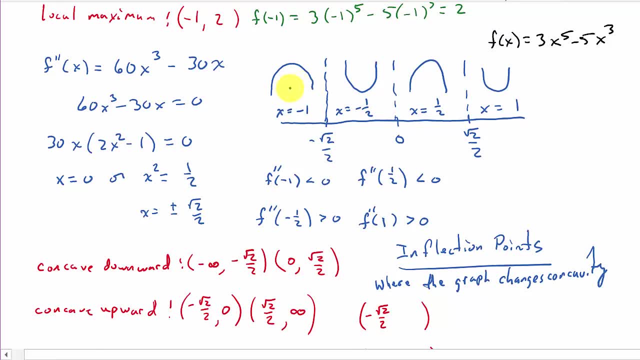 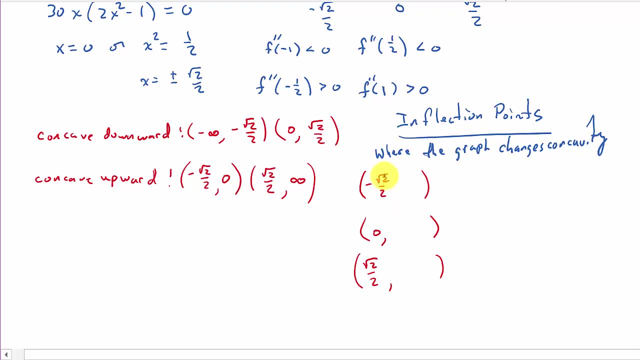 two over two, that's inflection points, because see it changes from concave down to concave up, concave up to concave down and concave down to concave up. all right, so how do we find the inflection, the inflection point? well, it's a point, so we've got the x coordinate. 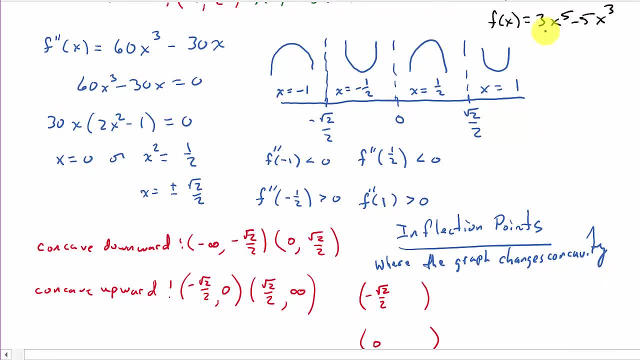 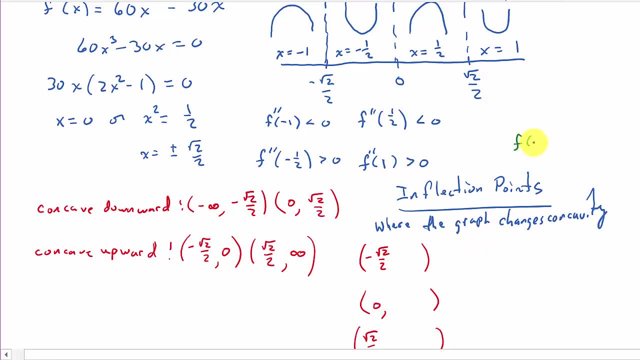 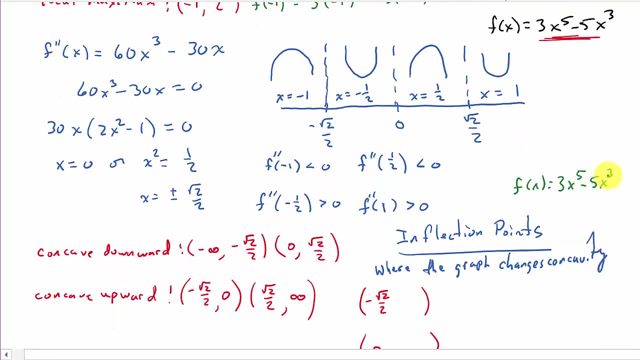 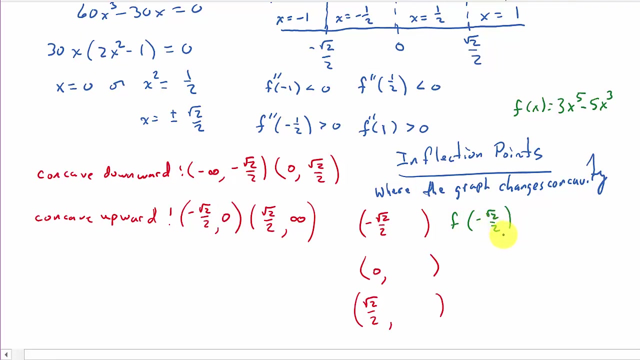 how do we find the y coordinate? we've got to plug it back into the original. so we've got f of x is equal to what, was that? three x to the fifth minus five x cubed. all right, so i'm going to write this: f of negative square root of two over two is equal to f of zero. well, 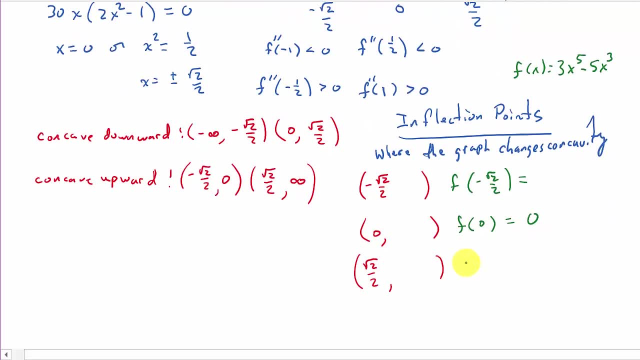 that one's easy: if we plug the zero in, we just get zero, and then we've got f of square root of two over two. so for these, you know you'll you'll need to punch these into your calculator. so, uh, i'll go ahead and do that and then i'll start the video back up when i get the answers. 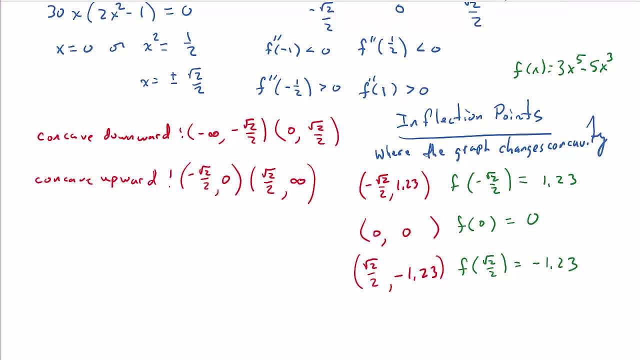 all right. so this is what i came up with. uh, assuming i punched it in my calculator, right i'm sure if i didn't, i'll hear about it in the comments. but anyway, there's your inflection points. okay, so you just take this, you plug it in for x here and here, punch it in your. 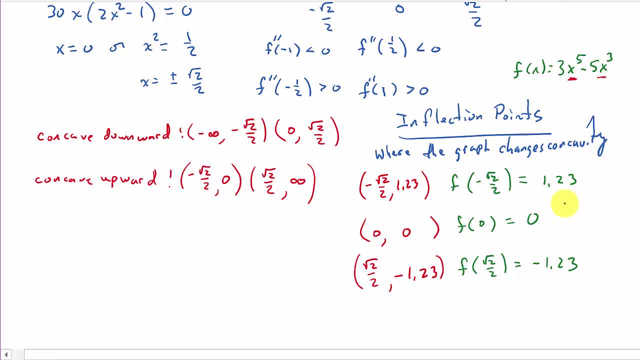 calculator and i believe this is what you should get all right. so now we found everything we've got increasing decreasing uh, local max min concavity and points of inflection. so now we need all this information in red and we're going to use that to sketch our graph. so i'm going to get rid of 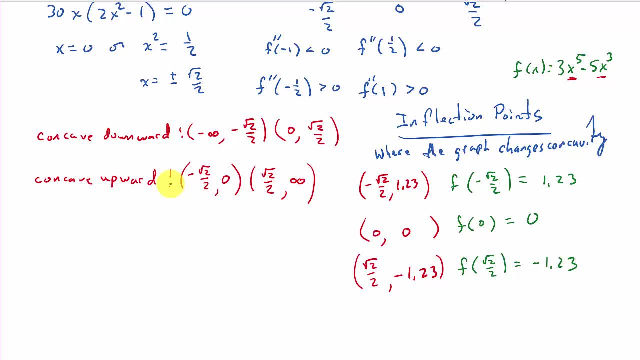 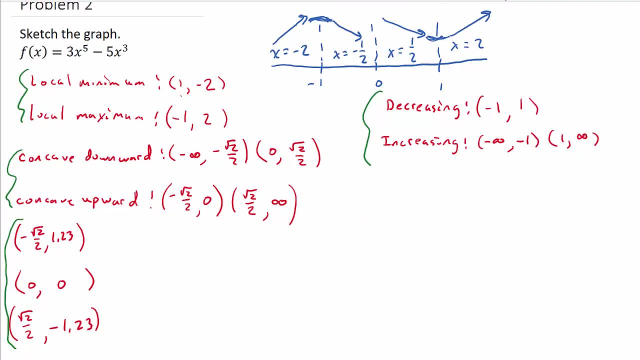 everything else except for the stuff in red, and we'll sketch the graph. and i'll pause while i do that, all right. so now, let's, let's sketch the graph. so let's draw our x- y axis. well, let's do it in black, all right. so the first thing i want to do is i want to plot my points so i can see that i've 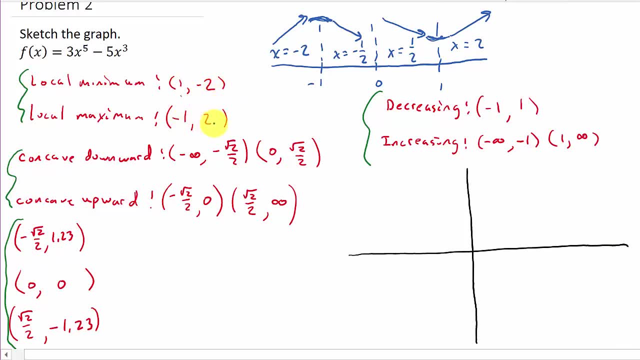 got one negative two, negative one, two, and then i've got these points to plot. so let's, let's do this one two, all right, so let's see one negative two, that's an easy one to plot. and then we've got negative one two. plot that one there. 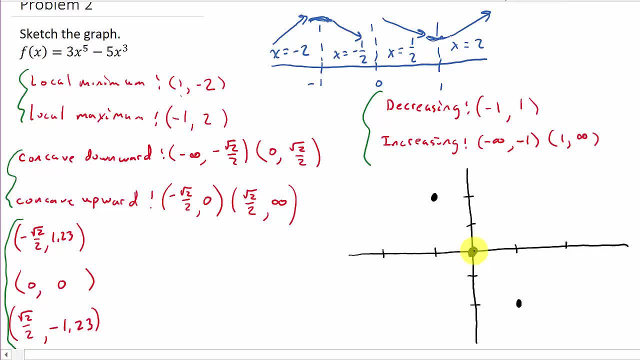 and then we've got zero, zero now square root of two over two and negative square root of two over two. remember, square root of two over two is was point seven something. so the negative would be negative 0.7. so that's going to be between one and zero, so that that point's going to be here. 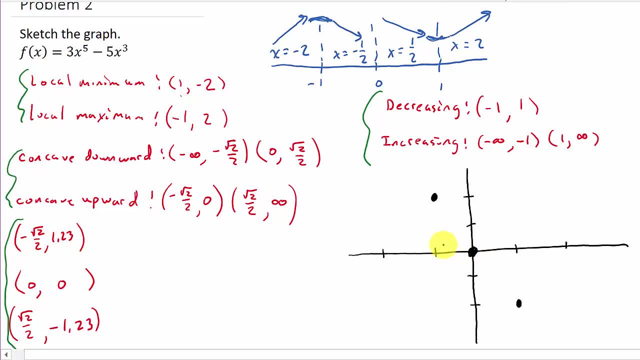 let's see, let's plot this one, so we're gonna be here and then we're gonna go up just over one, and then for this one, we're gonna go up just over here, we'll go to about right in here and then just below, and then just below, negative. 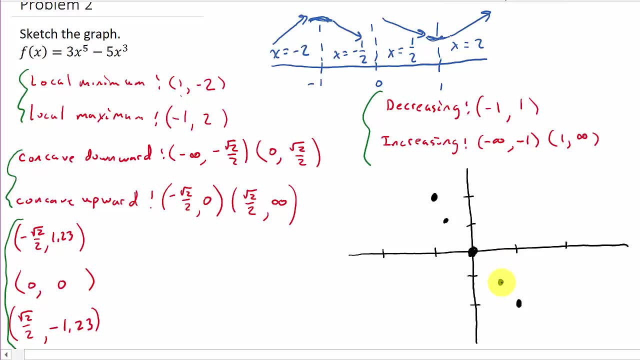 one like that, okay, and if you want to, you can. you can label the points, okay, alright. so now let's see how, how good we can draw this. and of course, you know, it's probably not gonna look as good, because the marks I've made here they're. 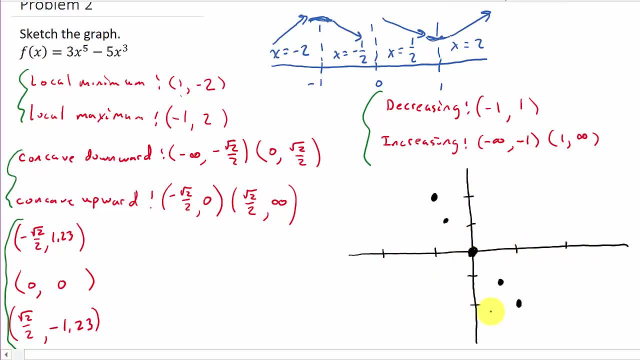 not evenly spaced. if you want your, if you want your graphs to look better, get you some graph paper and graph it on that, alright. so let's see what we have. so let's label this: negative: 1, negative, 2, 1, 2. alright, so let's see from negative. 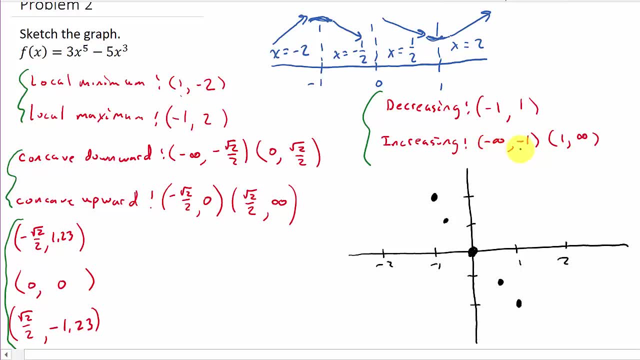 1, from negative infinity to negative 1. this thing's increasing so right down here. we know it's coming up like this, okay, so let's see it's increasing to here and let's let's check out the con cavity, so it's actually concave down, see this all the way to this point. so so that 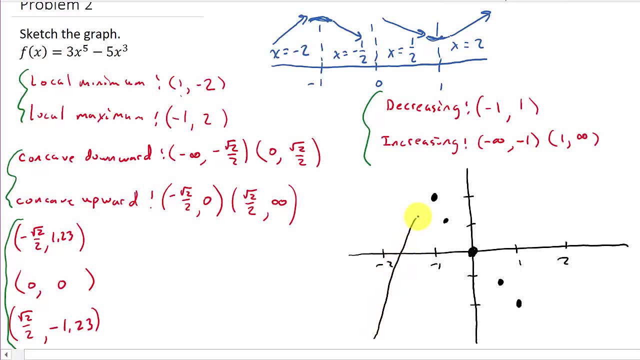 tells me it's gonna look like this and it's gonna turn and come back down, okay, and it's concave up. but look at this, from where are we from here? see negative square root of 2 over 2, that's these values right here and 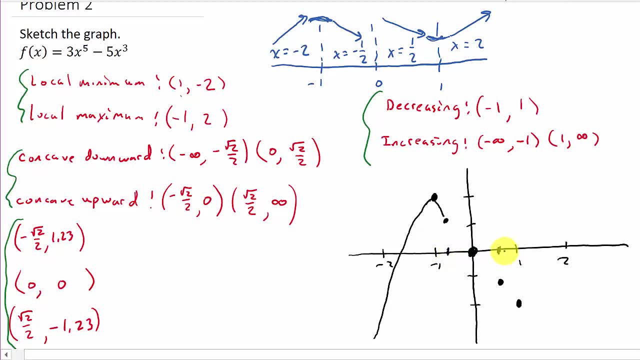 right here: negative square root of 2 over 2 and square root of 2 over 2. from here to here it changes to concave upward. so that means when I'm coming down through here it's gonna kind of do like this: I don't know if you can see and you know. 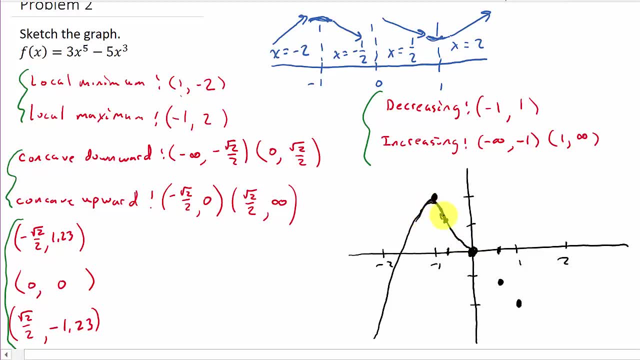 you might want to see it's. it's doing this, it's coming in like this and then it's kind of, and then it's changing to concave upward. so you got it, you got to show that. but then look at this: from 0 to square root of 2 over 2, see it's going back to concave downward, but also. 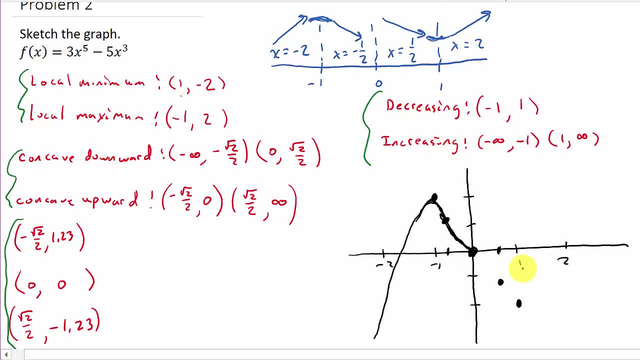 keep in mind this thing: from negative 1 to 1 it's also decreasing, so we know what's coming down. see, we're gonna have to come down to this point and turn back up, because from 1 to infinity it's increased and so when it gets here it changes concavity. so that means it's going to go. 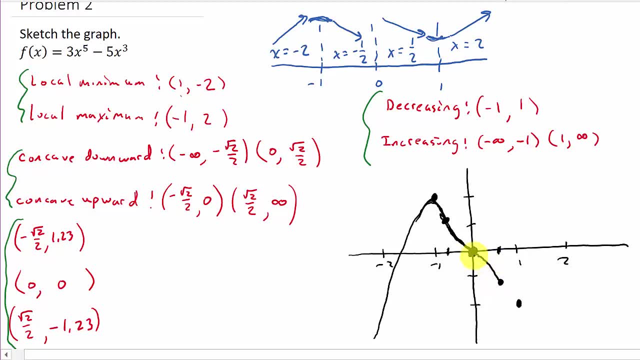 like this: okay, and then from square root of 2 over 2 to infinity- which is this point- it changes back to concave upward. so it's going to go, come back in like this, and I don't know if you can tell the exaggeration I have in there. but